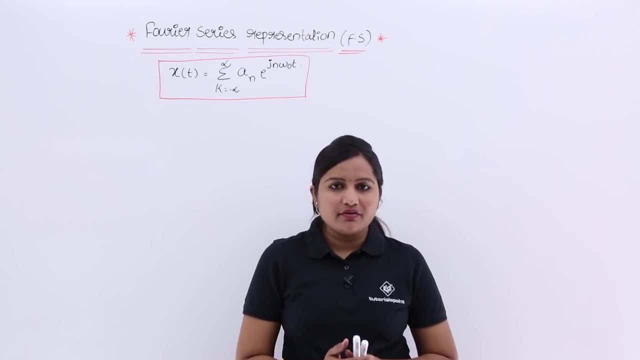 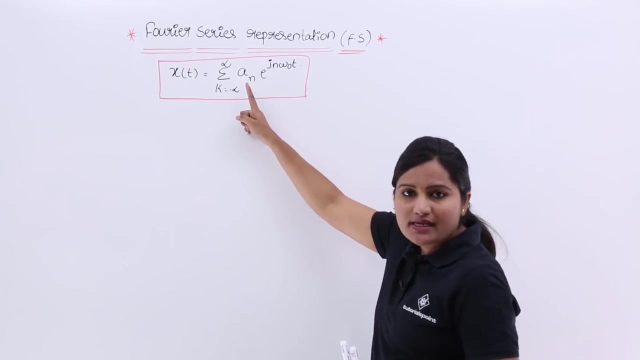 In this video I am going to derive Fourier series representation of any signal. So here, whenever you had Fourier series representation of any signal, you are going to get this equation in your mind. that is, x of t is equivalent to summation, k is equivalent to minus infinity, to. 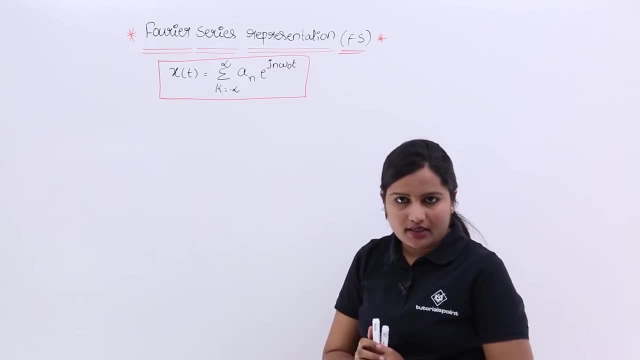 infinity, a n into e, power j n, omega naught t. This is the representation in Fourier series, Fourier signal x of t. How we are getting this equation. So now we are going to derive this equation for Fourier series representation of the signal x of t. First of all, before getting 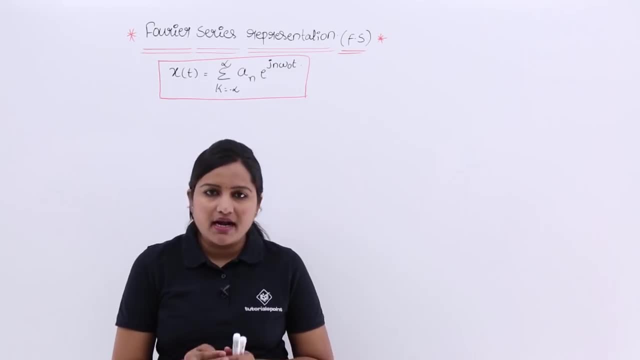 into this derivation. I want to discuss the periodicity of the signal x of t. Why? Because we are going to represent this Fourier series for periodic signals. So now our signal x of t is said to be periodic when x of t is equal. 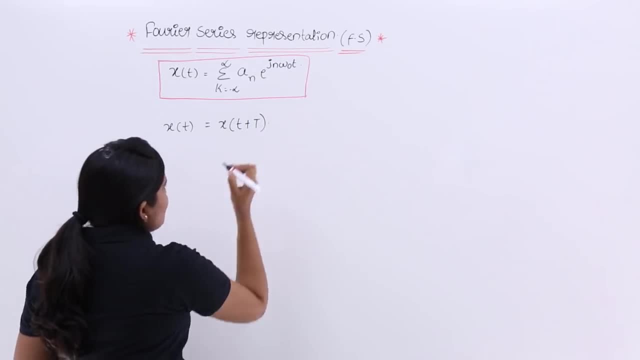 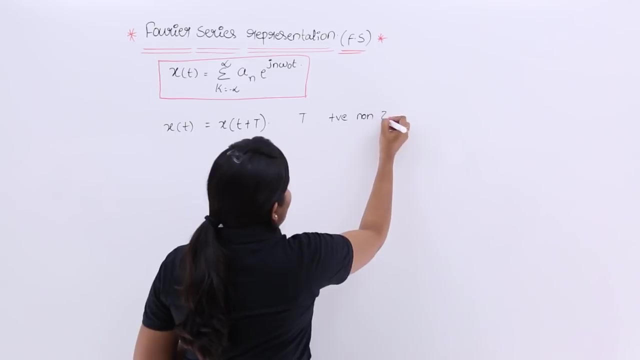 into x of t plus capital T. That means for every t interval of time the signal is repeating. then that is said to be a periodic signal. So always t is said to be positive and non-zero. So please keep in mind: So always t is positive and non-zero, That means whatever the value. 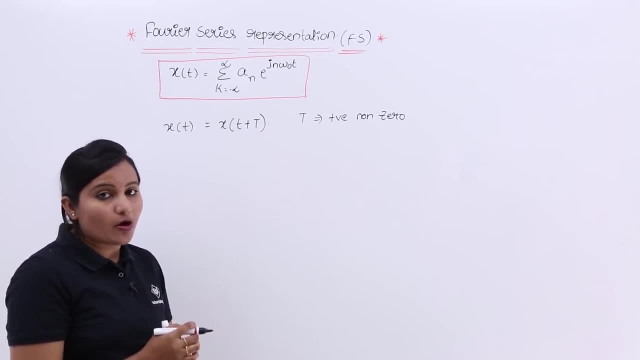 of t that is satisfying this condition. that must be positive and non-zero to say the signal is periodic signal. Now coming into the actual process. So here a signal is said to be periodic when x of t is equivalent to x of t plus capital T, where t is the fundamental period of the signal. 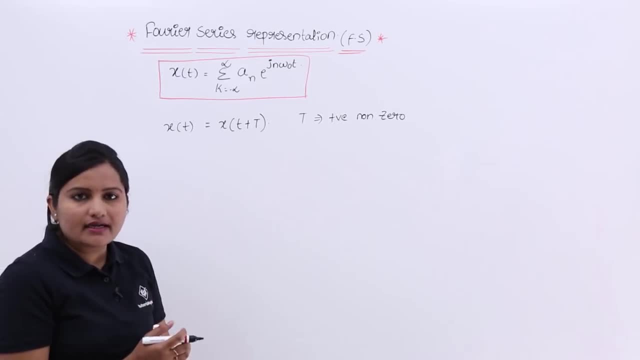 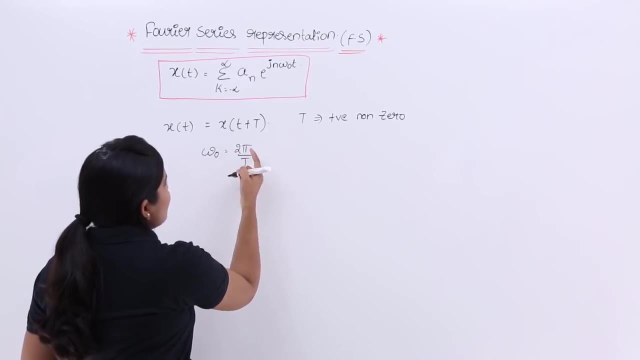 If you want fundamental frequency, then how we can get. fundamental frequency means: So omega naught is equal 2 pi by t. As you know that 1 by t is f, that omega is equivalent to 2 pi f. So generally omega is. 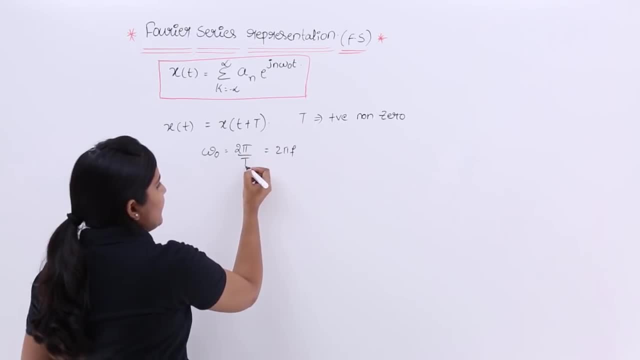 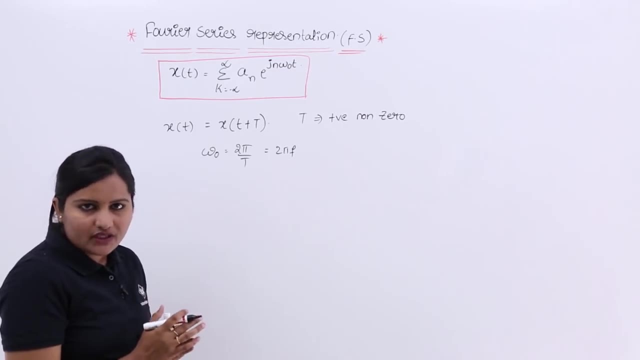 equivalent to 2 pi f. that is why I am writing in place of f, I can write 1 by fundamental time period. So like this, you are going to get the fundamental frequency of the signal. Now coming to the different signal, different periodic signals. if you consider, For example, x of t is equivalent. 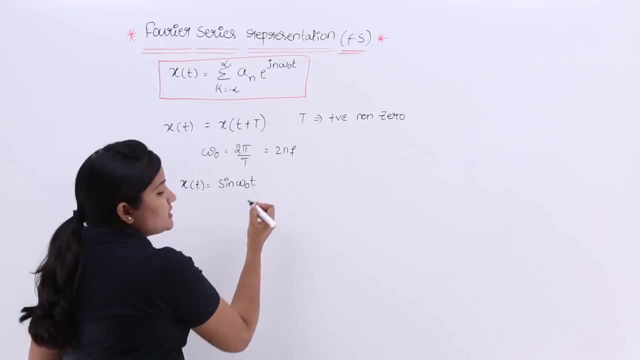 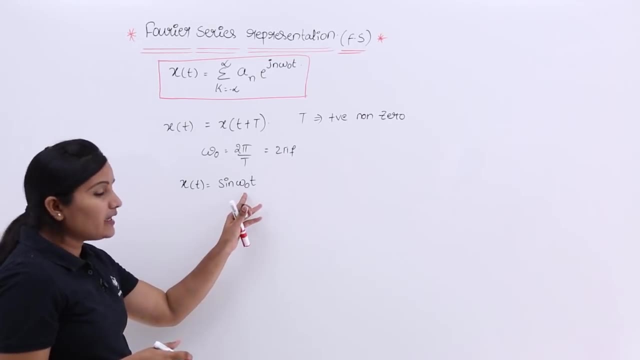 to sin omega, omega, naught, t. This is a periodic signal, So with some period, capital T and we are having another type of signals. This is just a sinusoidal signal, So and other type of periodic signals may be in complex form also. That means x of t is equivalent to e, power, j, omega, naught, t form. 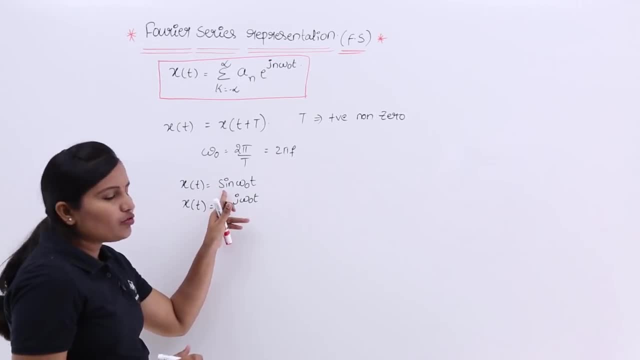 also. So, for example, if you ask to find out what is the period of this signal, how you can find the period of t. So you can find the period of t. So you can find the period of t. So. 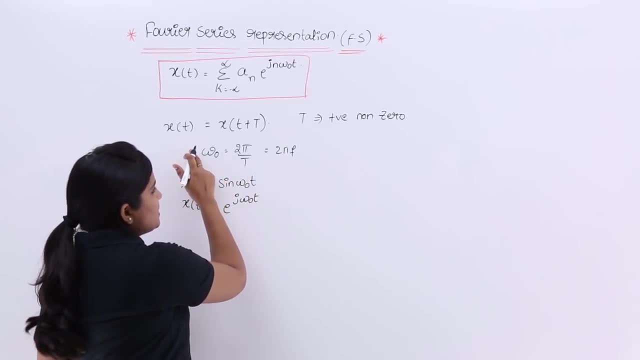 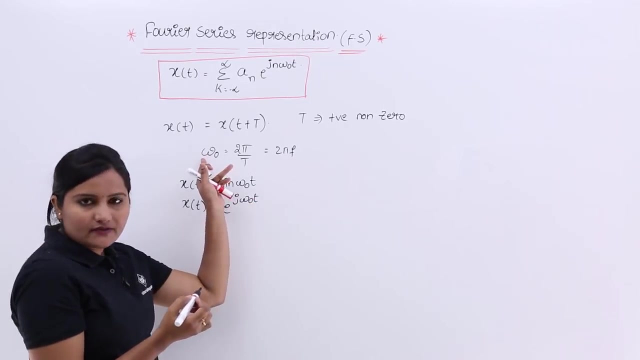 that signal means. So from this equation you are having, t is equivalent to 2 pi by omega naught. By taking 2 pi by omega naught you are going to consider the fundamental period of the signal. So here also, whatever you are having at omega naught, that can be considered as fundamental. 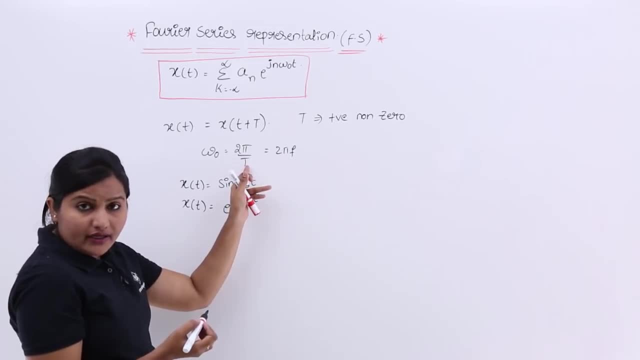 frequency. From that frequency, if you consider t is equivalent to 2 pi by omega, naught here also, you are going to get the fundamental period of the, your signal. So here, whatever it may be, either for the sinusoid or for this complex exponential, the period is. 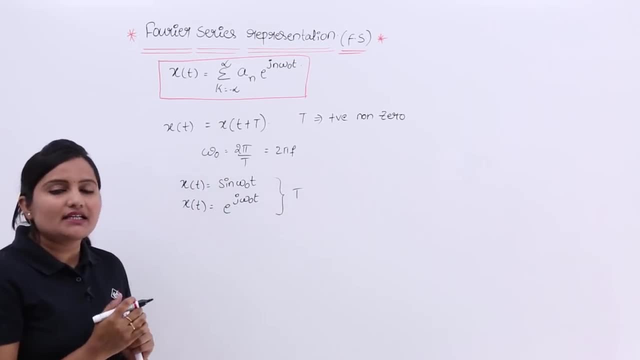 equivalent to t. The period we are having that is equivalent to t, For example. so which signal I want to consider is I want to consider a complex signal. If you are representing your series representation for a complex signal, then by using that equation you can represent any simple signal. 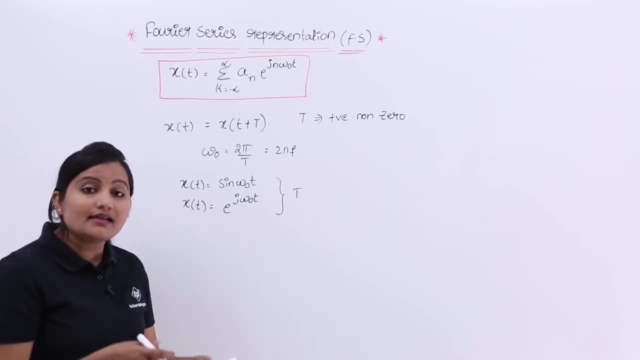 a complex signal. why? because this having both real and imaginary part. so, coming to here, this is having only real part. so if you represented both for real and imaginary, then obviously when you given for real or imaginary individually, then you can easily represent by that equation, that's. 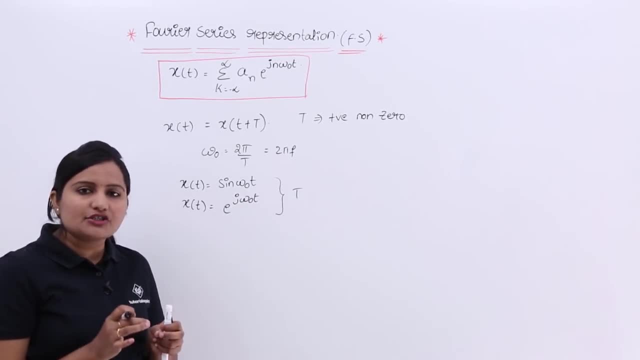 why i'm considering complex signal, complex continuous periodic signal. so one of the best complex continuous periodic signal is e, power, j, omega, not t. this signal i am going to consider as my signal to represent in fourier series representation. so if i consider this signal, so here i need to see for fundamental period. so this fundamental period of this signal is t. that means 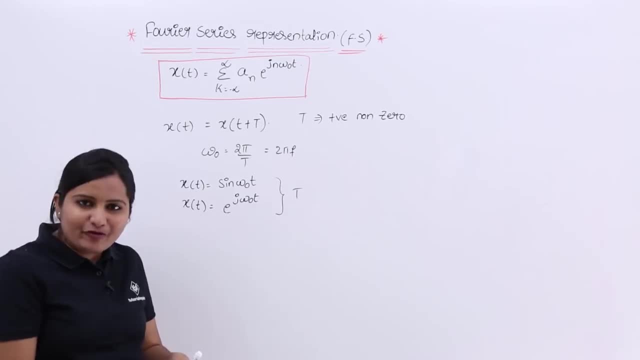 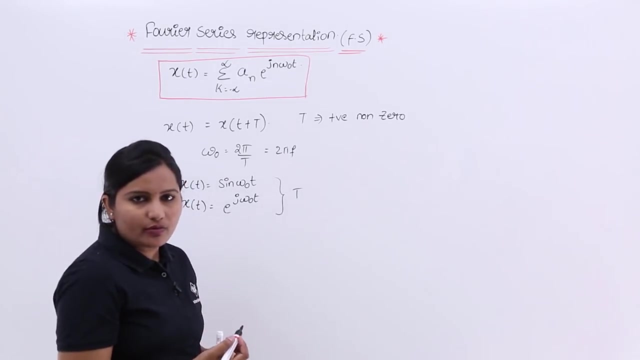 this exponential signal is keep on repeating for every t. so now if you are having uh, you know that exponential signal may change. that means the value of that exponential may change. so exponential is not only e power, j omega t. it may be e power j, 2 j omega t, 3 j omega t, like that you are having. so 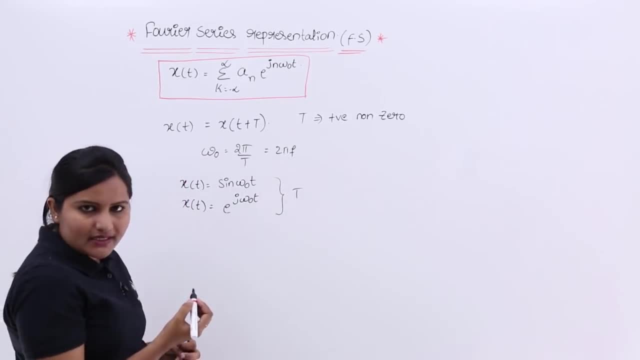 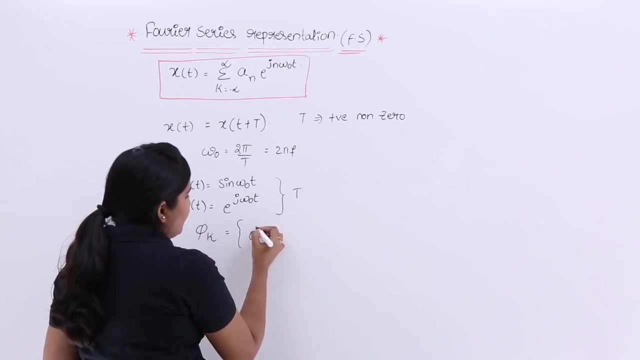 many exponential. that means. so if you want to represent, so, if you want to represent this set of the set of exponentials, then i want to represent that set as phi k. so phi k is equal to set of e power, j omega, not t. e power. so plus j omega, not t. j 2 omega, not t. so e power, j 3 omega. 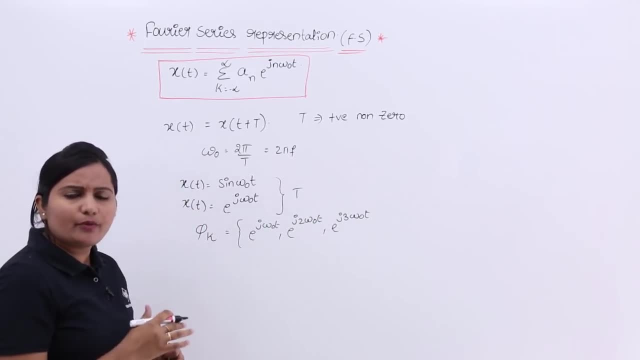 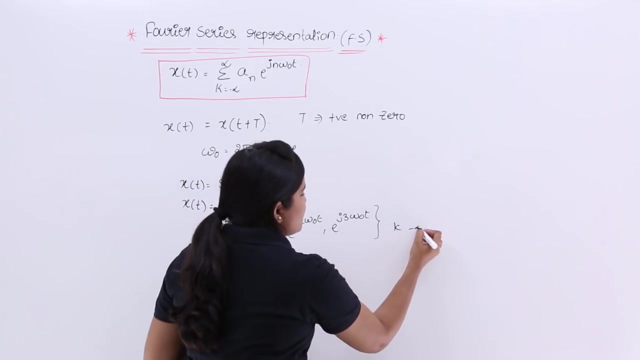 not t like that. i am having so many exponential in positive and negative power as well, as we are having so many exponentials, so that means k value starts from minus infinity to infinity. so whereas k value starts from minus infinity to infinity, that means it may include negative powers, also e power. 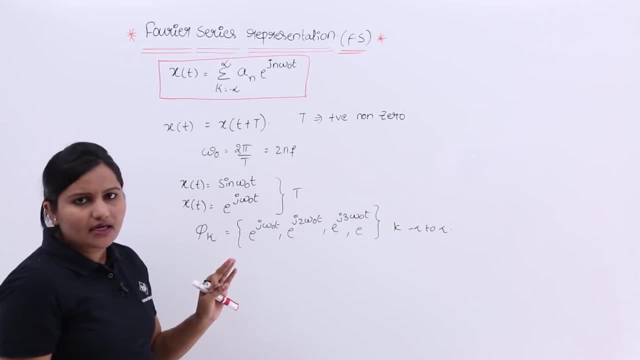 minus j omega r t, minus 2 j omega r t, minus 3 j omega r t. you are having so many exponentials, complex, continuous, periodic exponentials. so if you want to represent all that set how i am going to represent is i am going to represent with phi k. so this phi k, i am simply 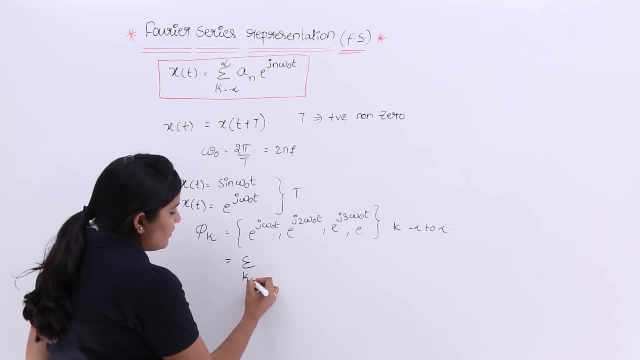 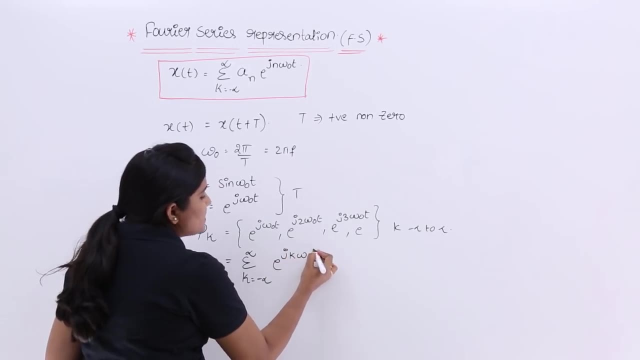 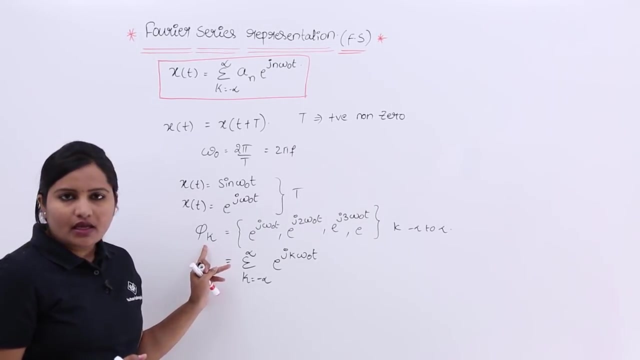 writing. like this: summation of k is equivalent to minus infinity to infinity. e, power, j, k, omega, naught, t. like this i am considering, if you want to consider like a set, if you want a linear combination of this set, if you want a linear combination of that set, if you want, if you want to consider the 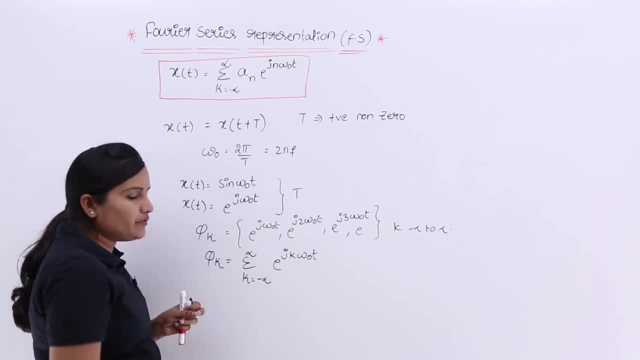 linear combination. i am going to represent that linear combination with phi k. that phi k is equivalent to summation, k is equivalent to minus infinity, to infinity, e, power, j, k, omega, not t. why i am writing like this? if you want to submit each and every continuous, complex, periodic. 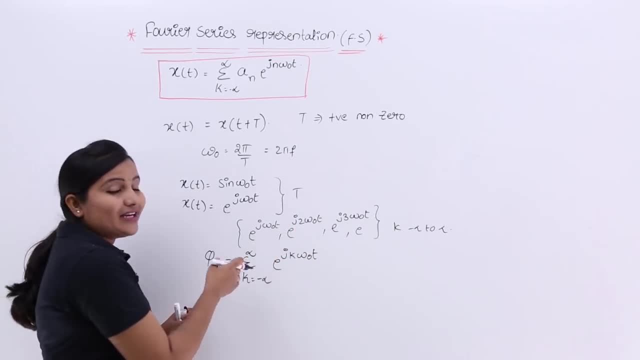 exponential in this set, then you have to write it like this piney and write it in another way. you need to cover each and every exponential. You can see: if you substitute k is equivalent to minus 1, it will cover c, power minus j, omega, naught, t. If you consider k is equivalent to: 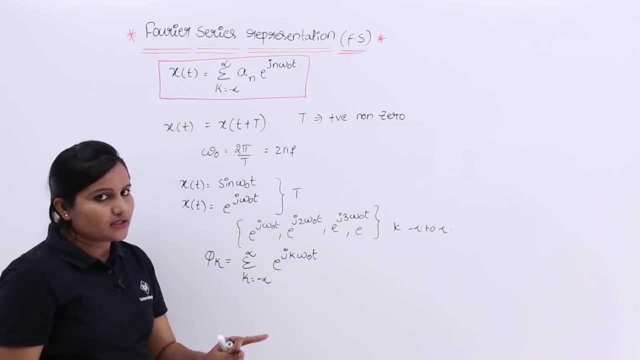 so it will cover c, power, j, 2, omega, naught t like that. if you substituted the range of k from minus infinity to infinity, it will cover total set of this exponentials. So now, so I am writing the linear combination like this, If you want to represent: 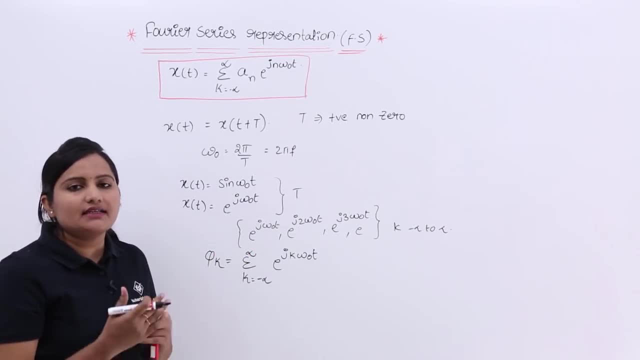 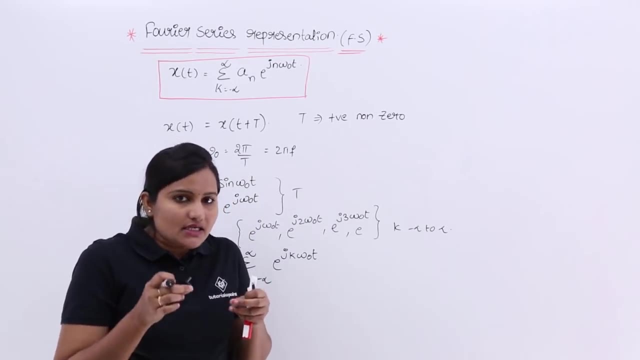 this linear combination with any signal. now we need to step out into the initial topics of signals and systems. So at the starting classes of signals and systems I given some important points about signals. So here always signals will follow vector analogy. So that means 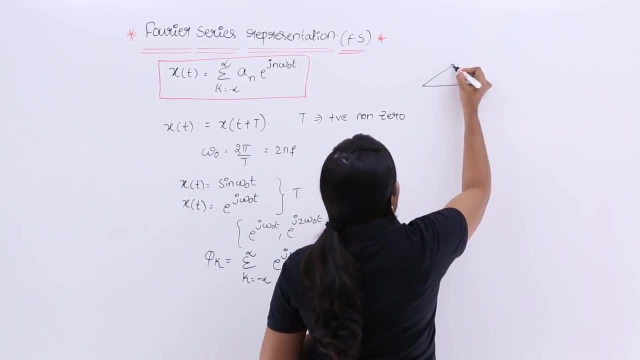 for example, if you want to represent any vector- v 1- in terms of v 2, we need to draw a perpendicular bisector And you need to trace the component of approximation from v 1 to v 2. then if you want to write v, 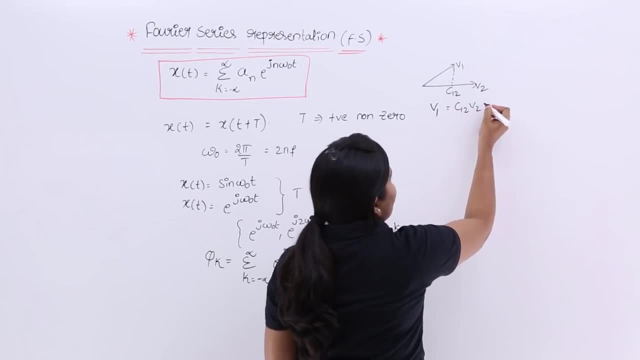 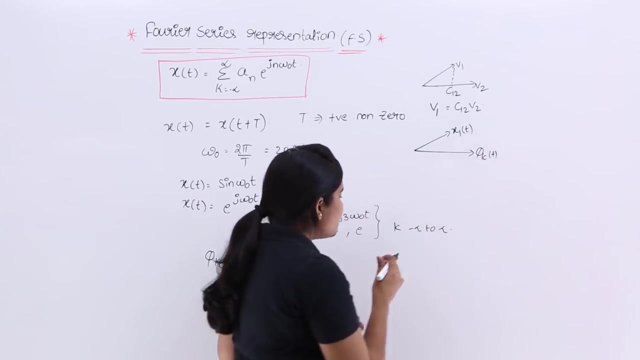 1 in terms of v 2, then you can write c 1 to v 2.. So this is vector analogy. Same analogy we are going to apply for signals. that means so here, for example, if you want to represent any x 1 of t in terms of this set phi k of t. So this is also a summation of signals. 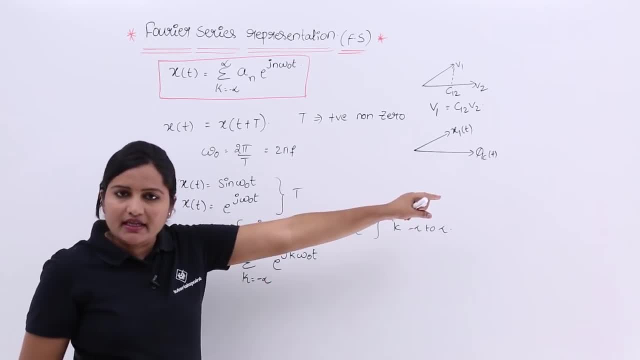 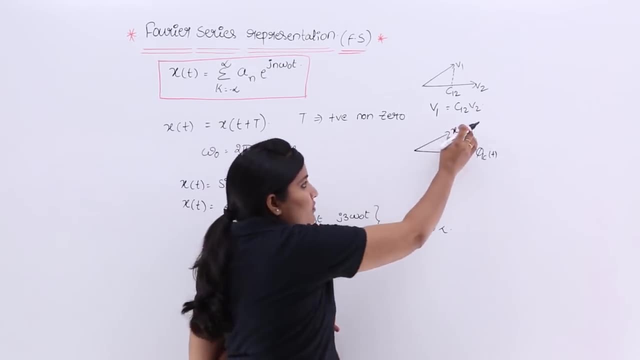 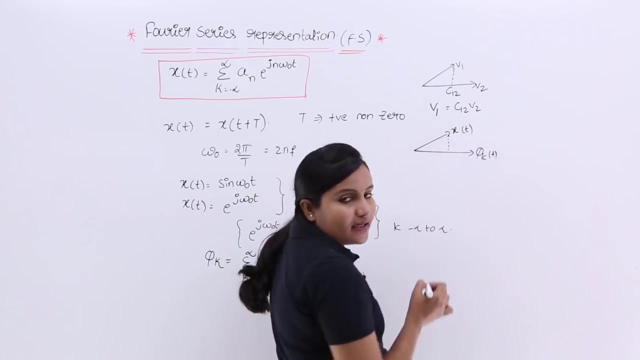 is also a resultant signal. So this set is also we can consider as this linear combination of this set also we can consider as a resultant signal. If you want to represent any signal x of t with respect to this set, you need to consider a perpendicular bisector here And I am representing that perpendicular bisector as a k. 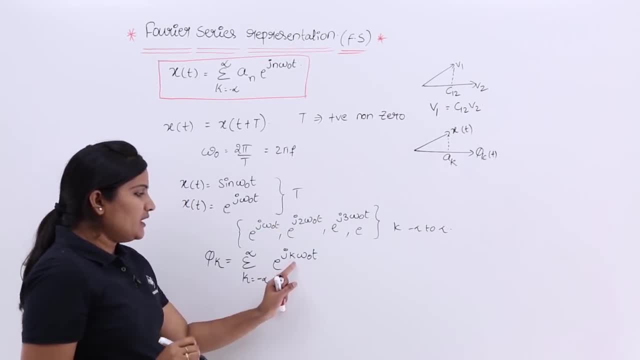 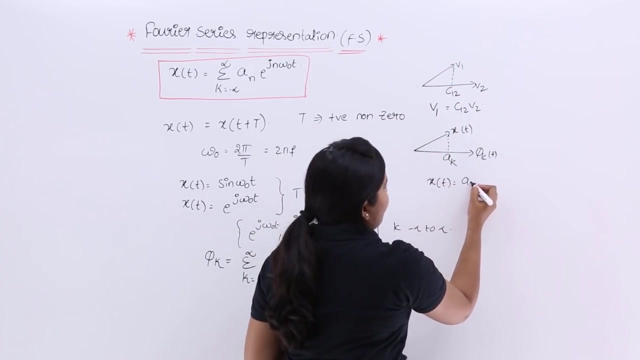 Why? because I consider in terms of k everything I considered in terms of k. that's why I consider a k, phi n, j, n. in terms of n, you can, you can consider a n, So that suffix is your wish. I considered as a k. So now, so, according to vector analogy, if you want to write x of t, how you can write a k. 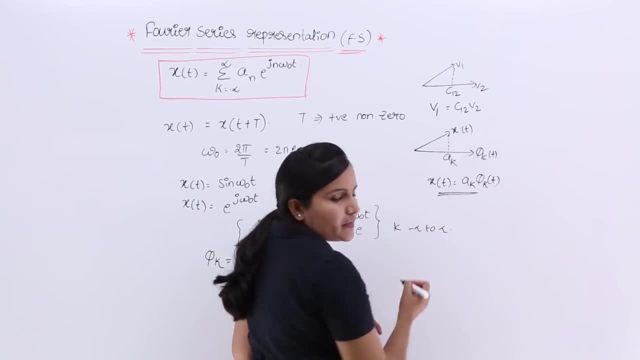 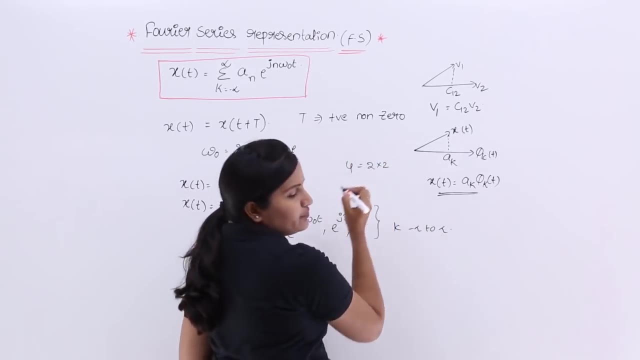 into phi k of t. like this you can write. So this is simple. if you want to write 4 in terms of 2, how you can write 2 into 2. whatever 2 is there, you can consider that as coefficient. For example, 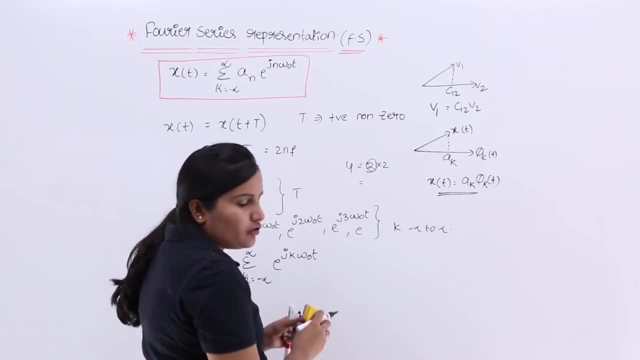 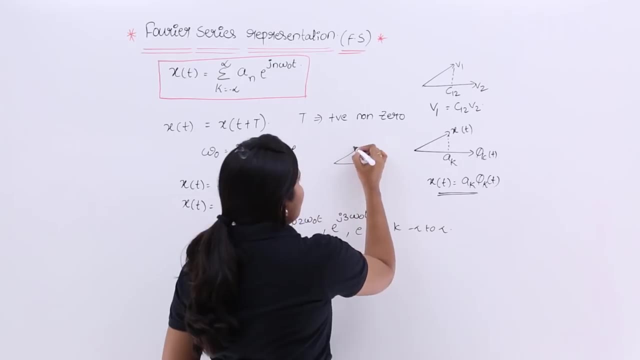 if you want to write, if you want to write same thing, if you want to write 2 in terms of 4, how you can write. So, for example, if you want to write 2 in terms of 4, how you can write means: 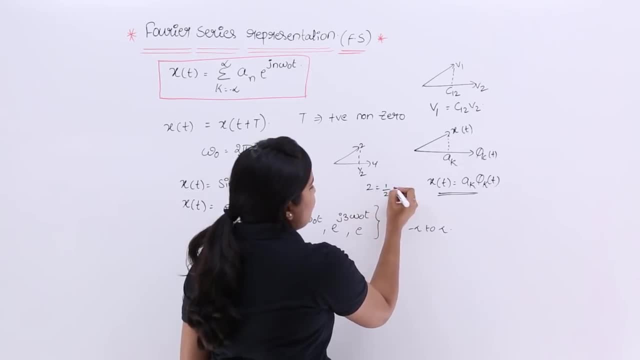 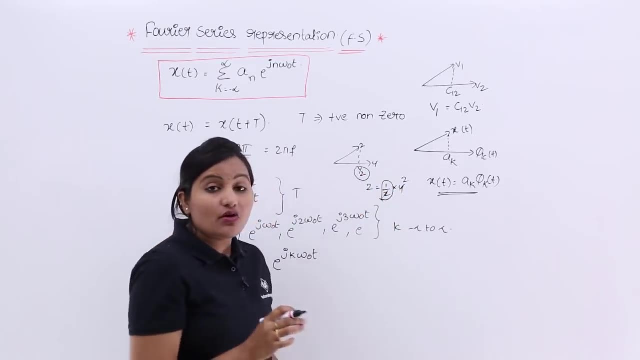 you need to consider 1 by 2.. So 2 is equivalent to 1 by 2. into 4, 2, 2s, 4.. So 2 equivalent to 2. whatever 1 by 2 we are having here that is called as coefficient of approximation and that is used. 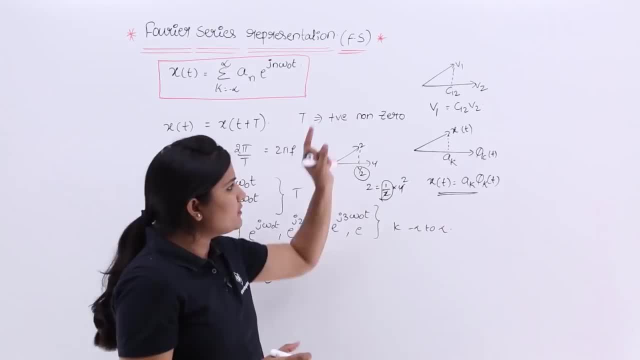 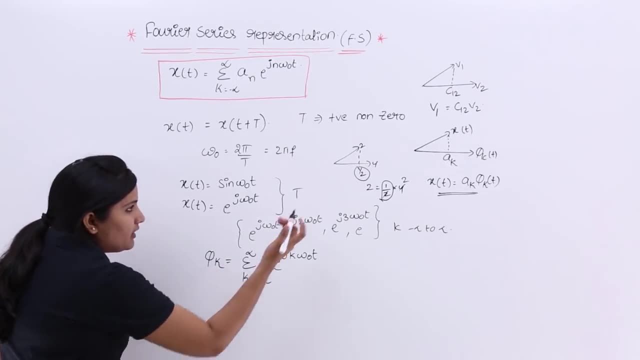 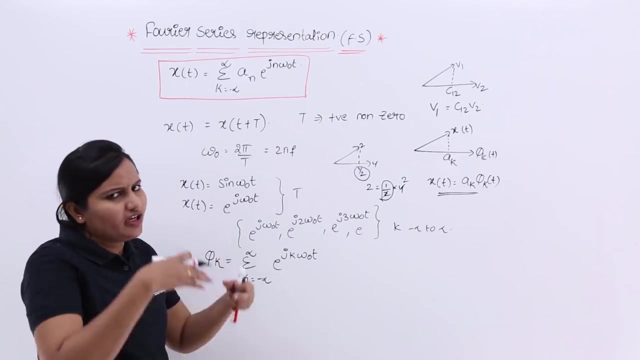 to approximate two different values. that is general process for vectors as well as signals. So, based on the theory, we can write: So: phi k, x of t. any signal, any signal in space that is called, that may be x of t or y of t or z of t, if you want to represent with this set. 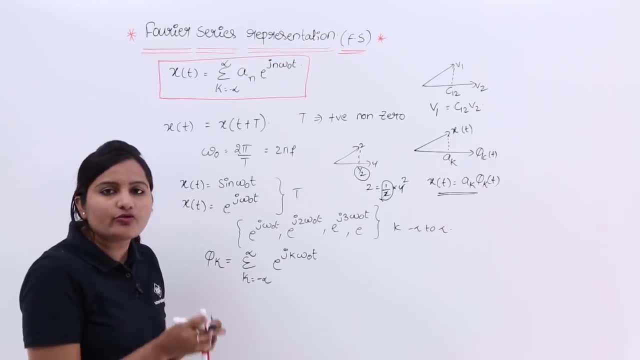 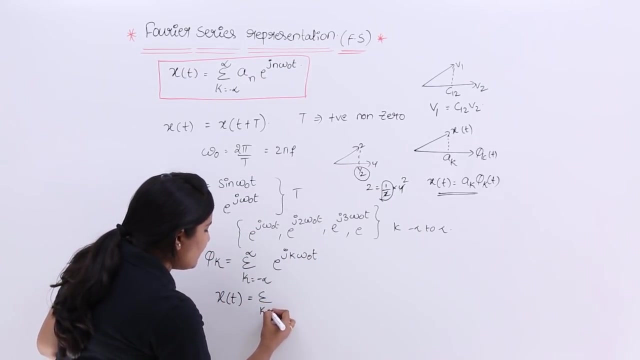 you need to consider, Consider an approximation coefficient. So that is here. I want to represent any signal x of t in the space with this set, with this complex exponential set. So now I want to consider that a k coefficient, So k equivalent to minus infinity to infinity, a k into e power, j k omega. 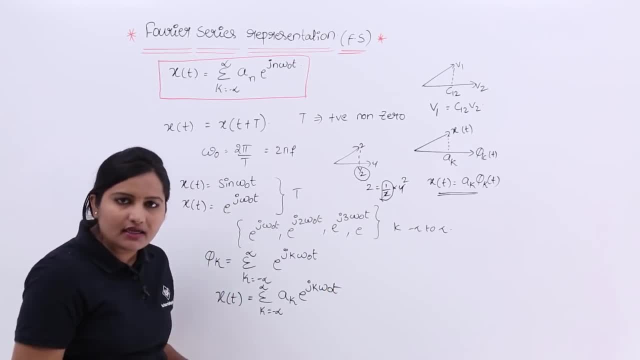 naught t So I can represent my signal. if I want to represent my signal with any complex exponential set, then I can represent like this: this is nothing but Fourier series representation of a periodic signal x of t. So now here, if you want exact representation, you need to find out a k. 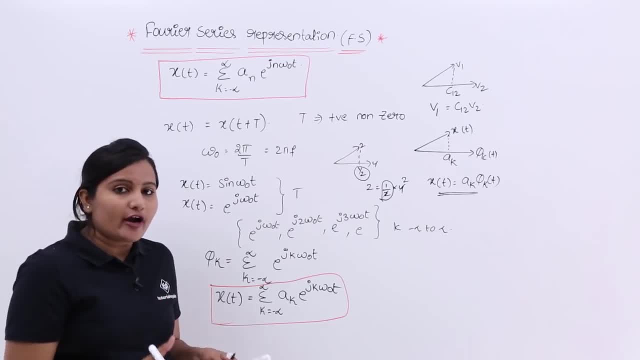 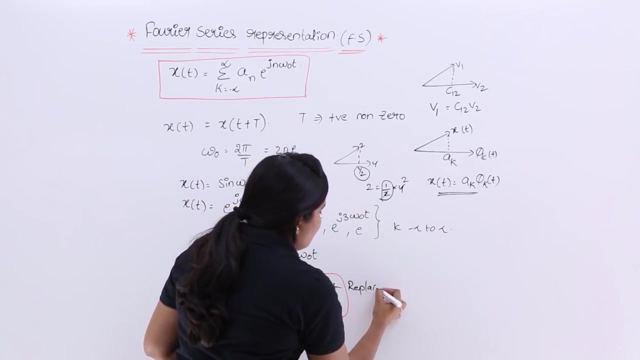 value. that we will discuss in the next class, how we need to find out the value for coefficient, For example. here this is the standard formula. So in so many text books you are having n, x suffix. So just replace k with n, then you are getting same thing. So here, summation k is equal. 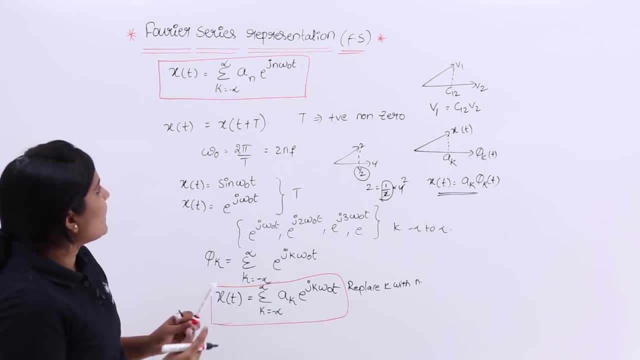 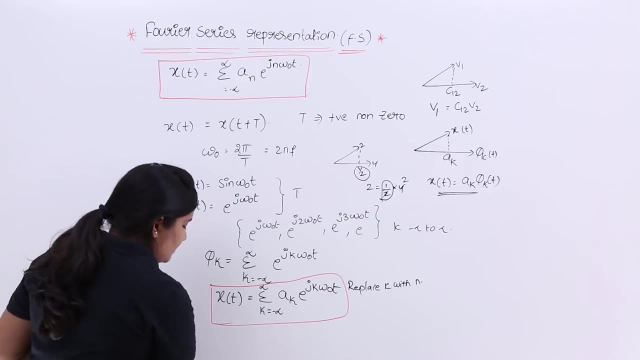 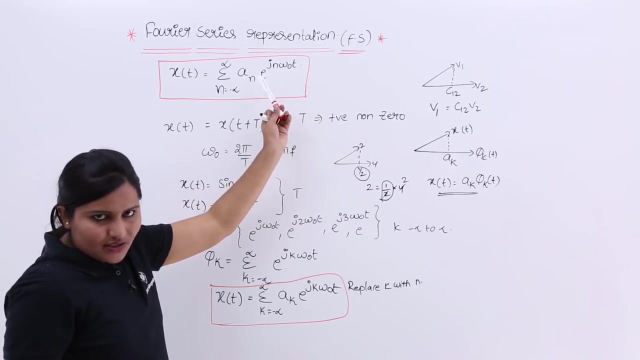 to minus infinity to infinity. So here n, you can consider n. whenever you consider n here, then you are getting n here. So n is equal to minus infinity to infinity. a n into e, power, j, n, omega, r, t. This is the standard formula. So here this is your derived formula. 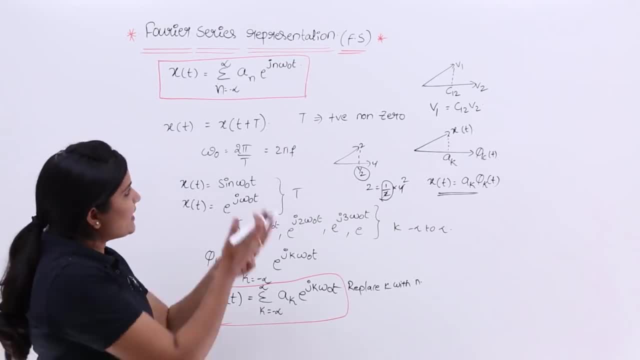 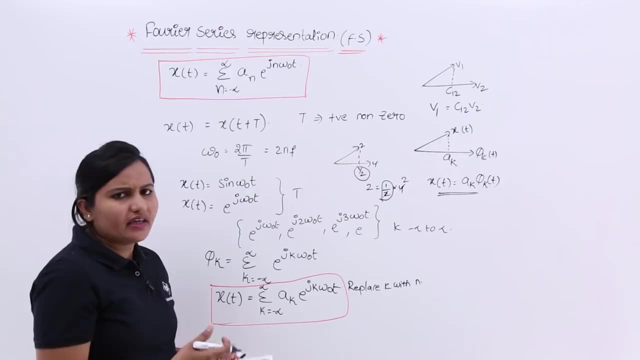 in place of k. if you consider n, you are getting same thing. Considering of suffix is not a matter. you can consider any suffix, not n, k, l, x, y or anything you can consider. the process is this. That means so you need to consider a complex periodic exponential set to reach. 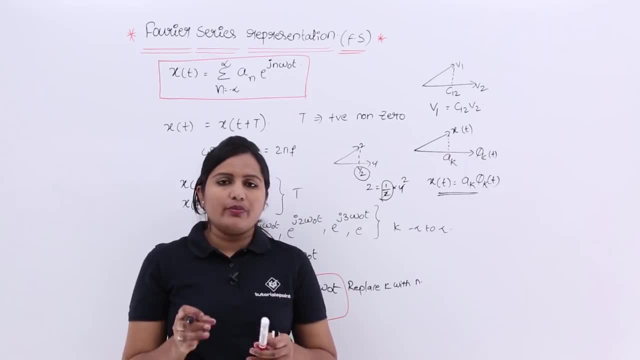 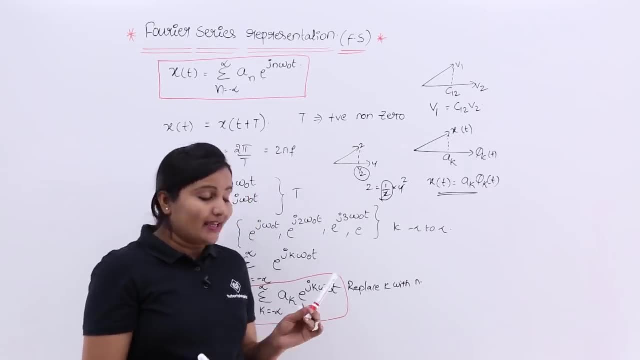 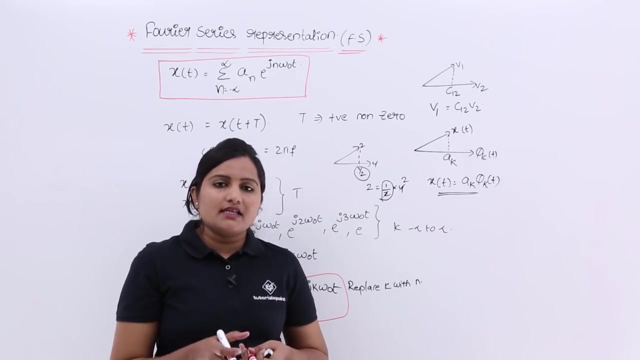 represent any signal in the space. So obviously. so, finally, what is meant by a Fourier series representation means representing any signal, any unknown signal, with the known set. That means with complex exponential set, summation of linear combination of complex exponential setting. That means, finally, you can frame the definition for Fourier series like Fourier. 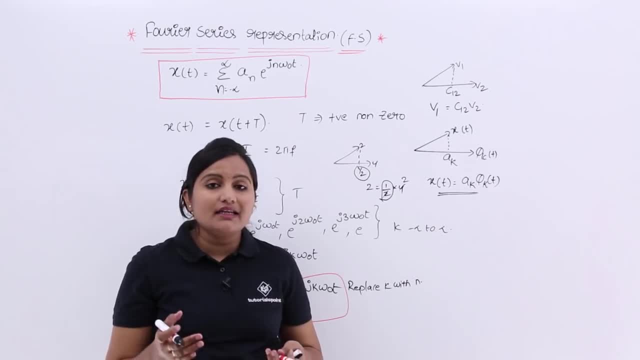 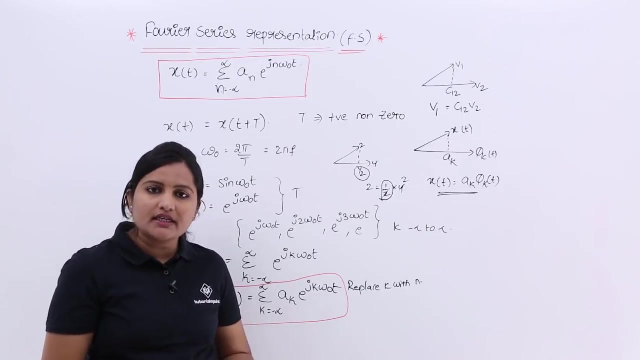 series is the representation: Representation of signal with linear combination of continuous, periodic, complex exponential set. So this is about Fourier series representation of the signal. in next class we will deal with the quotient. So by knowing the quotient and substituting in this formula, you are going. to get the exact representation of the signal. 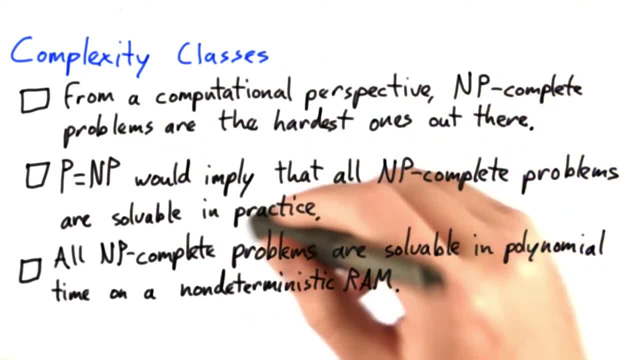 Let's take a look at a few questions about complexity classes, And I'd like you to look at these three statements and check which ones you think are true and leave unchecked the ones you think are false. So the first one is from a computational perspective. 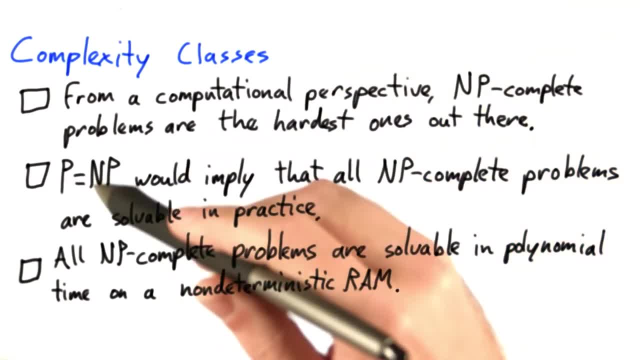 NP-complete problems are the hardest ones out there. Second one is P equal to NP, would imply that all NP-complete problems are solvable in practice. And finally, all NP-complete problems are solvable in polynomial time on a non-deterministic RAM.